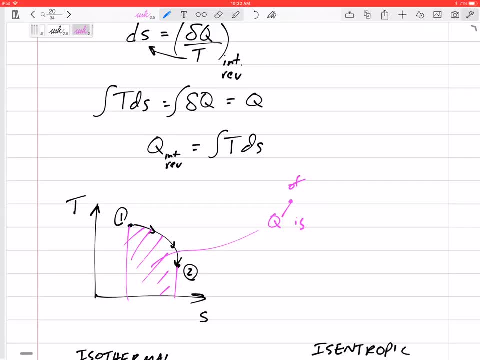 The Q of the internal, The Q of the internally reversible right, Q is sorry, Q is the internally reversible heat transfer. It is the area under the TS diagram. Alright, Q is the area under the TS diagram. So let's think about the TS diagram for. 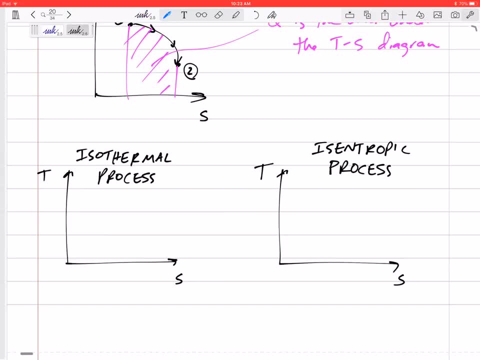 An isothermal process. An isothermal process, what would it look like on the TS diagram? Well, the temperature stays constant, So whatever temperature is at, it stays there. Maybe entropy is increasing, But the Q would be this area under the curve, which is a rectangle for an isothermal process. 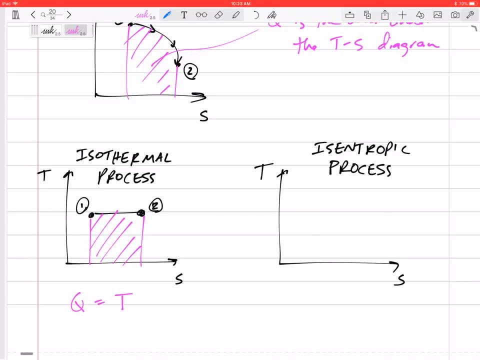 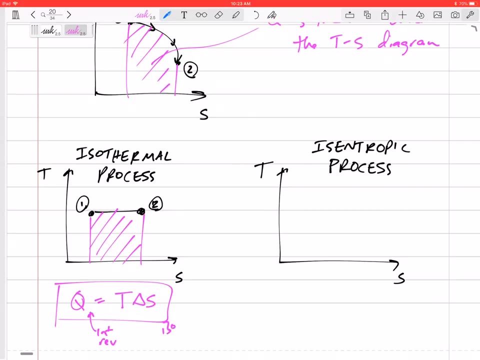 Q would be temperature, So it would be temperature times delta S for internally right, internally reversible Q equals T delta S, And again, that's only for isothermal. What about an isentropic process? What does that look like on the TS diagram? 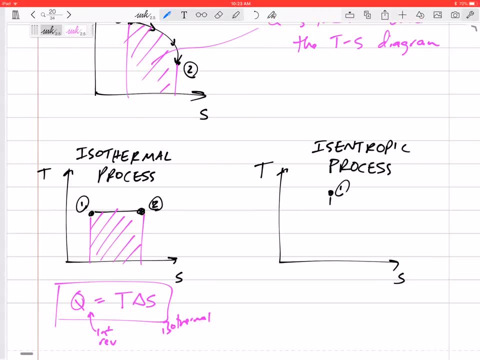 Well, if it's isentropic, maybe it starts here and it goes down to there, or up to there, Um, But entropy stays the same. What was? Is the area under the curve? for that? Uh, nothing. So Q is zero. 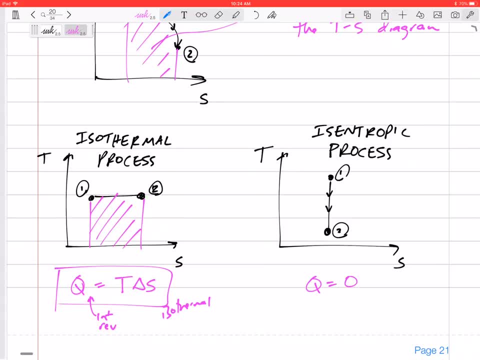 But we already knew that Um Q is zero for- And this is the internally reversible Q. We already knew that if we're talking about reversible and isentropic, then we know it's adiabatic. So that's just another way to show that it's adiabatic. 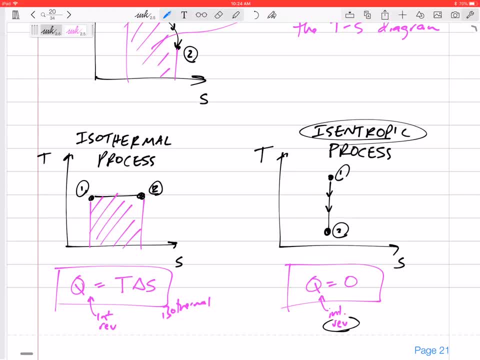 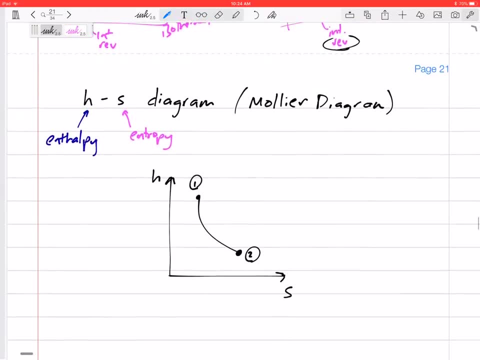 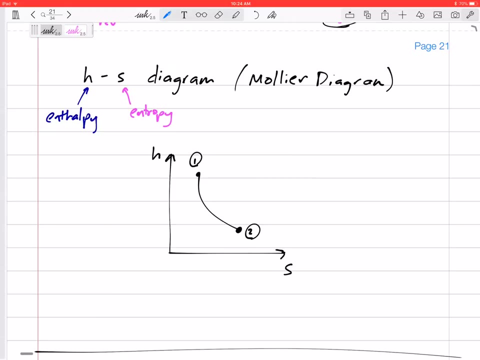 So these TS diagrams are interesting, And finding the area under the TS diagram gives you the value for the internally reversible heat transfer. Now another interesting diagram is the Moliere diagram or the enthalpy-entropy HS diagram. So for the HS diagram. 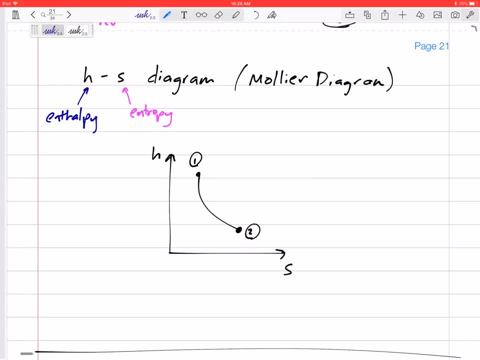 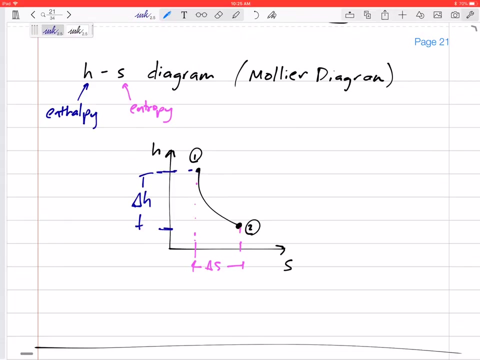 what these can kind of show. Um, here's our change in H: right, Our delta H is on this axis. And our Here's our delta S is right here. Right. Change in H. change in S. So this change in H is sort of a measure of. 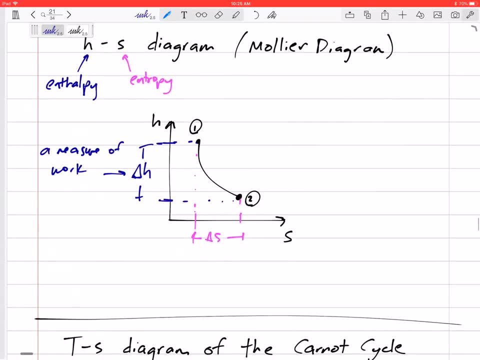 work. Our delta H is a measure of work And our delta S is a measure of irreversibilities. Our delta S is a measure of irreversibilities. So this diagram kind of shows you know, and you can compare different, you know paths. 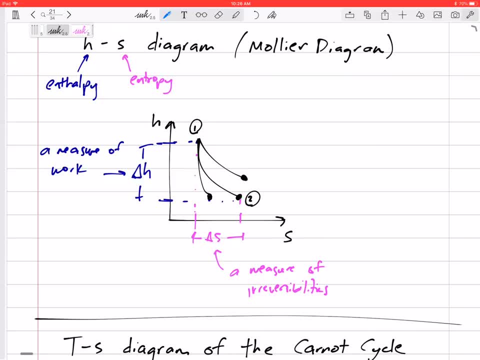 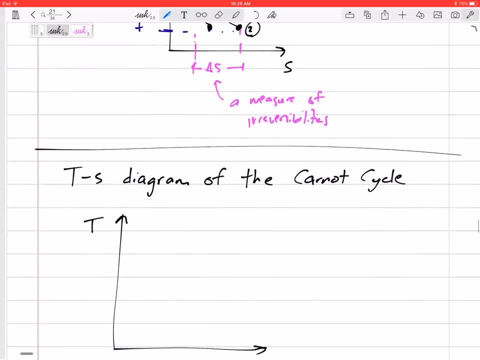 uh, which paths have? which paths have more work, which paths have less work? which paths have more are more irreversible? or which ones are more reversible, which ones are closer to the Carnot, the theoretical limit? Alright, so here's the TS diagram of the Carnot cycle. 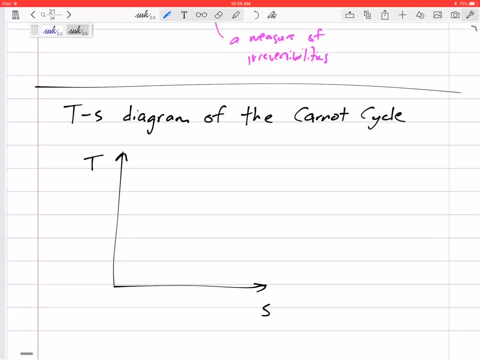 So we've done the PV, I believe. diagram of the Carnot cycle. If you remember that, it looks something like this: this, this, this, um. but I think the TS diagram really shows why the Carnot uh. 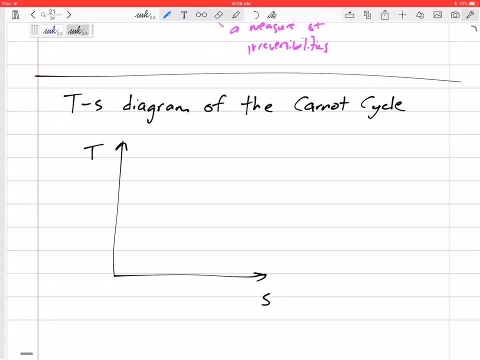 is the best. it's the ideal cycle For the Carnot cycle we had. we started at state one and we had an isothermal uh Q in isothermal process. Then we actually have an isentropic. 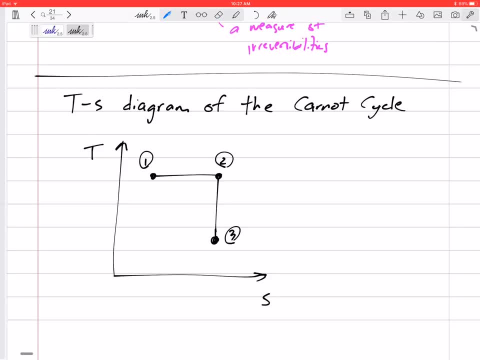 uh process to state three and then an isothermal process to state four and back isentropic to state uh two. And what did we say? We said the area under the TS diagram is Q. So from one 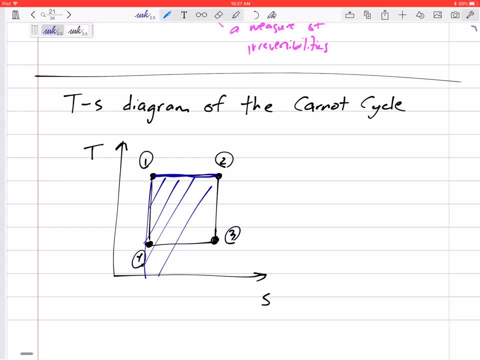 to two. the Q would be this whole rectangle, QH would be this blue, the QL would be from three to four. that would be this green. QL is this green and the difference in the two would be the work. 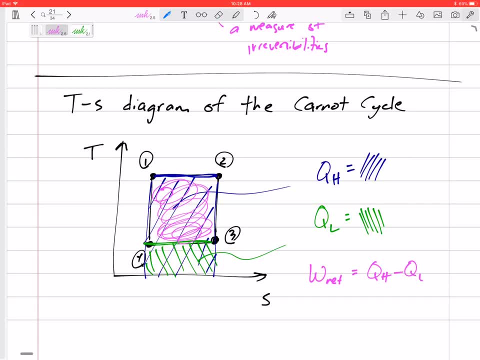 Work would be QH minus QL, which is this, you know pink area on the chart. So that's what's a. that is what a Carnot cycle looks like on the TS diagram. Alright, So, uh, section six, it's, it's. 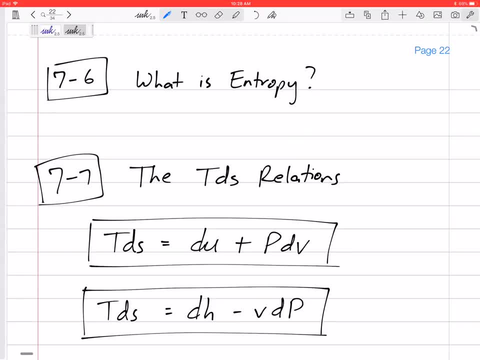 kind of interesting. I think it's a funny um little paragraph in the book. uh, but entropy, let's just say it's really molecular disorder. It's really molecular disorder. It's, it's a. you know, it's a. 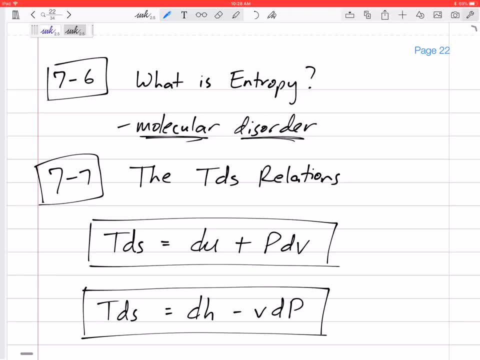 measure of disorder. uh, and if you it's really, it really goes down to the molecular level which we won't get into in this um class. Alright, seven, seven, real quickly, is just the TDS relations. 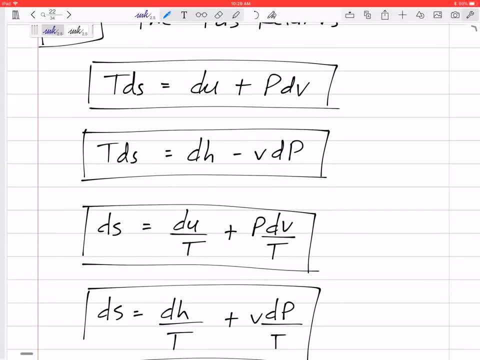 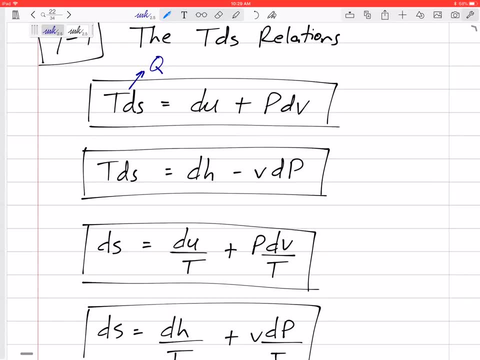 uh, you could, we could, we could derive these, um, but it really comes from the fact that this TDS is Q and this PDV is work and this DU is. is just that DU? Alright, So we're. 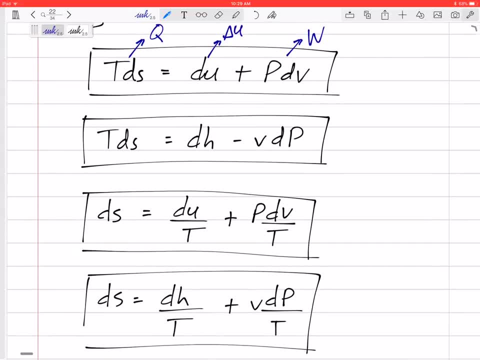 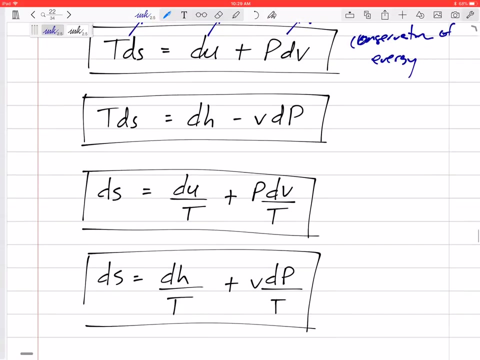 just gonna uh have these um four relations, these four equations, uh, so that we can use later. They come from conservation of energy. They come from conservation of energy, And so these are relations, so we have equations for uh. 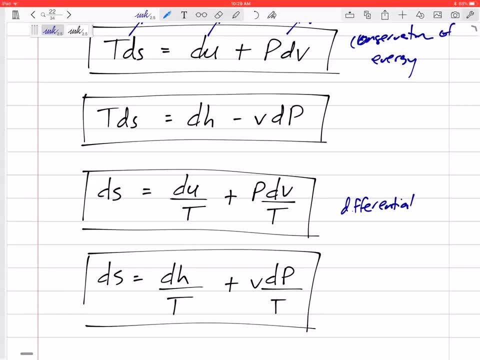 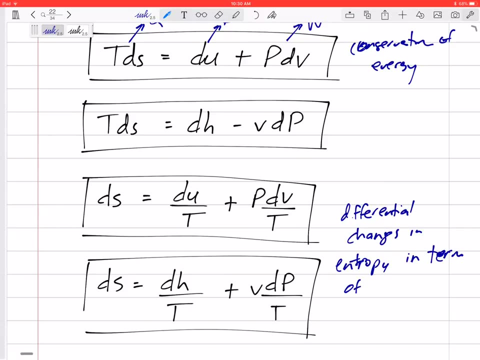 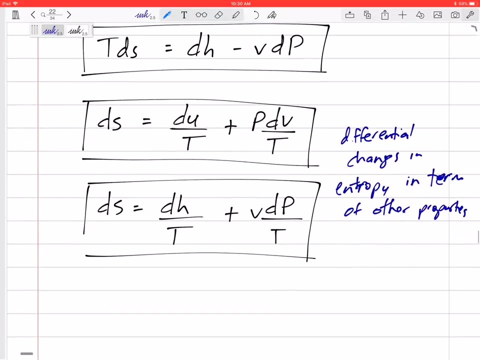 differential changes in entropy and we have this DS in terms of other properties, In terms of age and pressure and temperature, and DU. Okay, Alright, so, uh, we're gonna take this and you, you know that DU uh T. 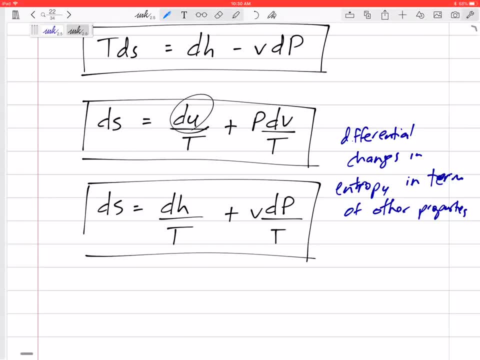 sorry, uh, DU is really C CV, right, And DH is really is related or not exactly, but it comes from specific heats And DH is CP. so we're gonna take that and go to 7-8 and 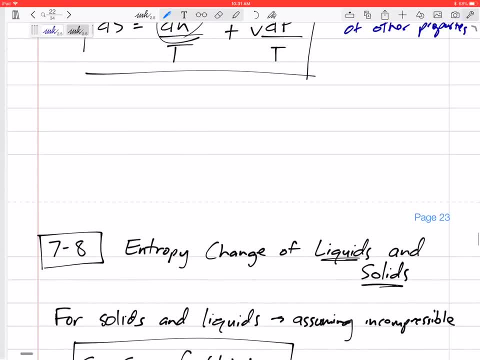 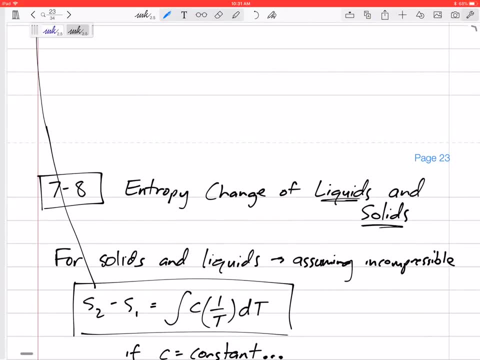 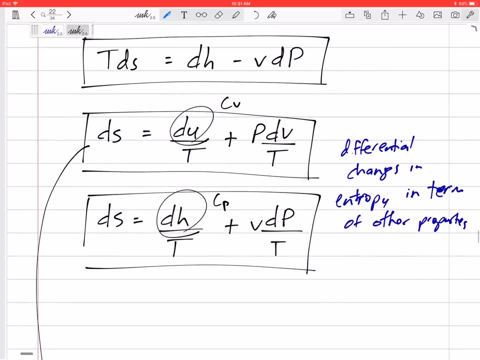 talk about the entropy changes of solids and liquids. So we can take, uh, this equation right here, this DS equation- and I'm not going to do the derivation, but I think you can see it- For solids and liquids. we're going to assume that. 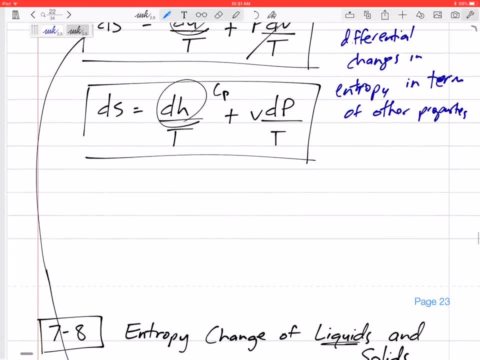 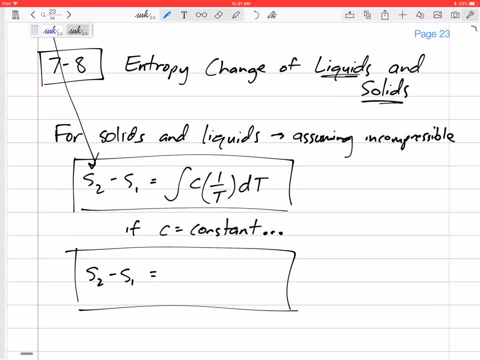 it is incompressible, And so DS is equal to DU over T and substituting for uh specific heats. that, and taking the integral of both sides, S2 minus S1, is equal to the integral of C 1 over T. 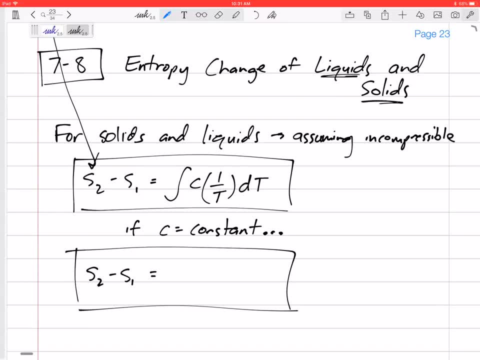 DT Integral of C 1 over T DT. And if C is constant, we can take this out of the equation and we can get C at some constant or average temperature. and what's the integral of 1 over T DT? It is ln of. 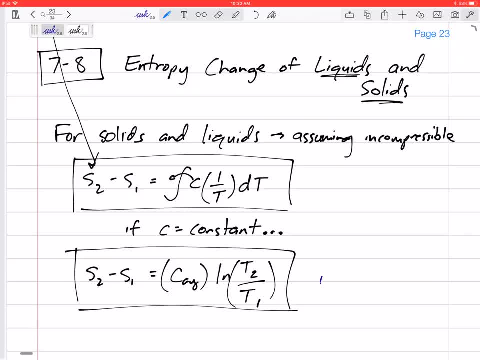 T2 over T1.. So now we have an equation for the change in entropy using specific heats and using the temperatures. This is for uh, solids and liquids. So either this is more accurate, um, but if we so, if we have an equation. 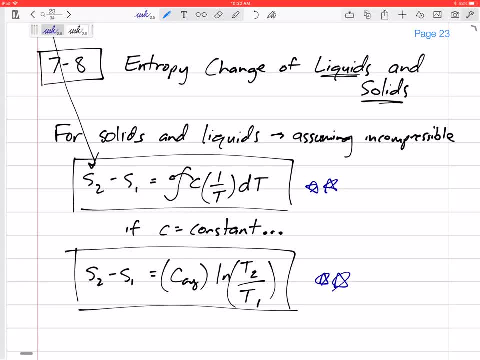 for C. we can use that under the integral um or we can just assume that C stays the same, or we can see the change in C from one temperature to the next temperature. take the average uh. take the C at the average temperature. 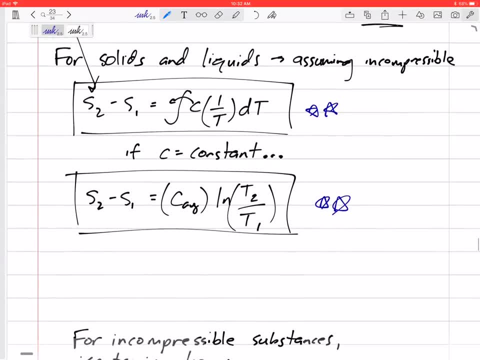 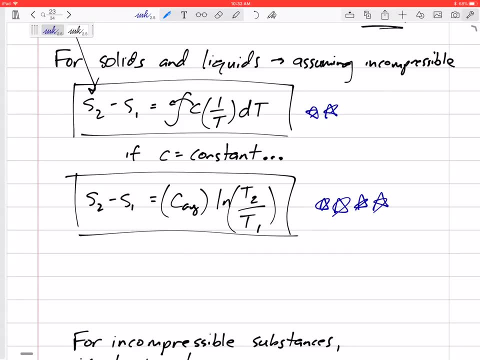 use that times ln T2 over T1.. So here that that's the main point. right here We've got an equation for change in entropy for solids and liquids, um using the specific heat C value. Just a note, uh. 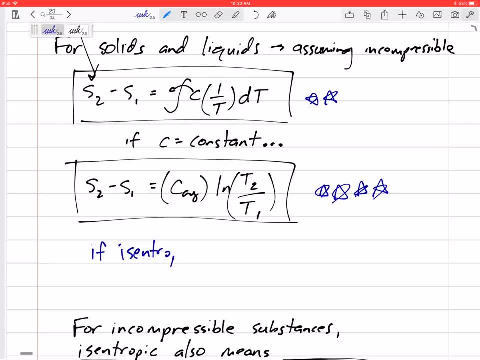 just look at this equation. If the process is isentropic, then what does that mean for this equation? If it's isentropic, this side of the equation, the equation is zero, And so you know, divide that C to the other side of the equation. uh, 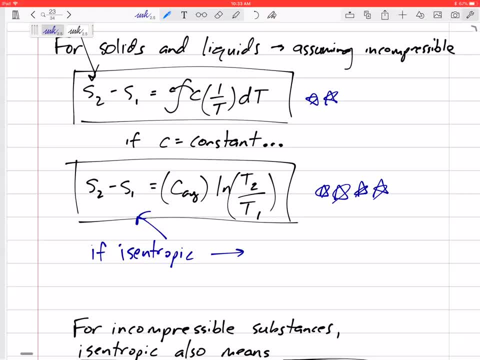 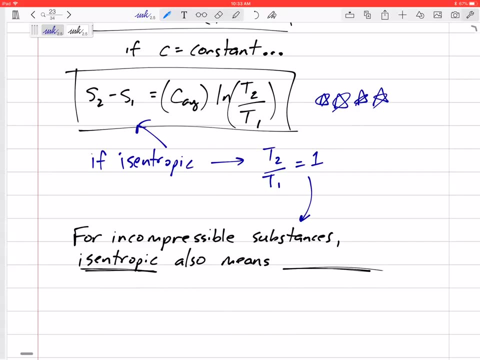 when is ln zero? ln of one is zero. So if it's isentropic, T2 over T1 is equal to one. So for incompressible substances like solids and liquids, isentropic also means isothermal. Alright, so there's just a note. 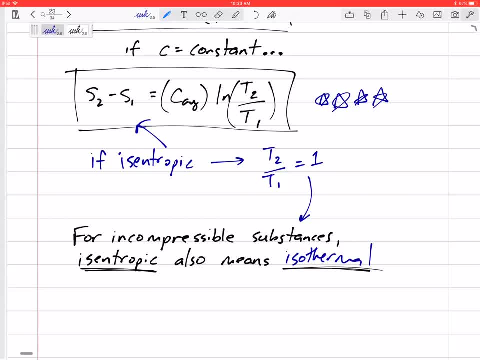 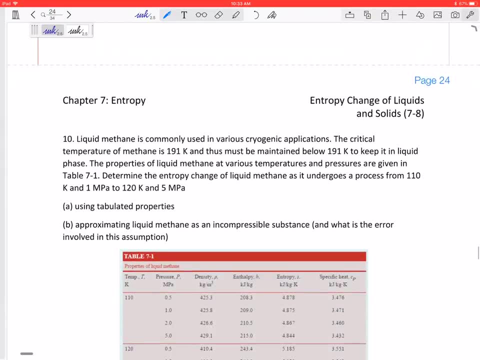 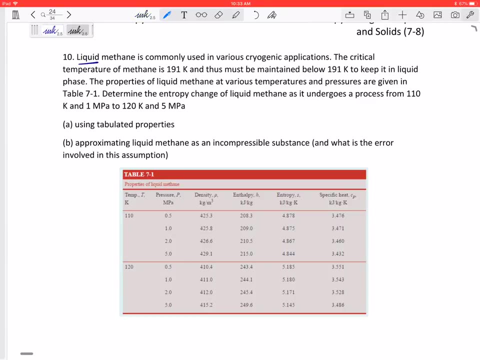 something to note. Solids and liquids- um, if it's isentropic, it's also isothermal. Alright, let's look at one solids and liquids problem. Uh, liquid methane, Uh, it's commonly used in various cryogenic applications. 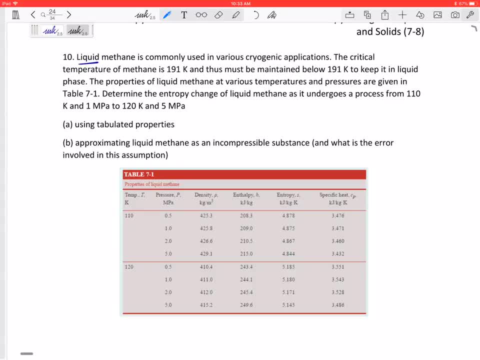 Critical temperature is 191 K and thus must be: must be maintained below 191 Kelvin. keep it in liquid phase. The properties of liquid at various temperatures are given in the table. Determine the entropy change as it undergoes a process from 110 Kelvin. 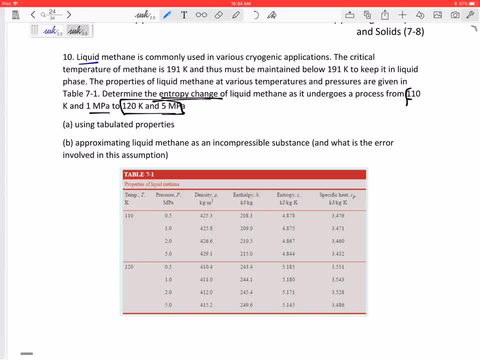 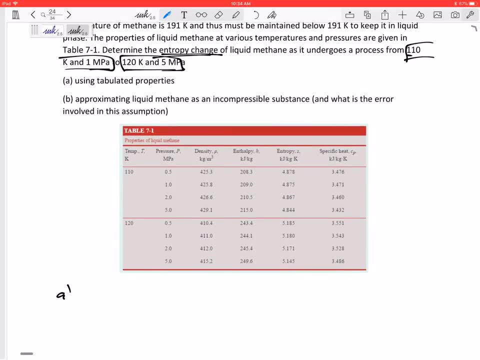 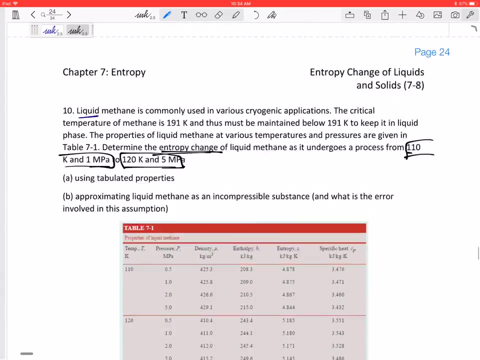 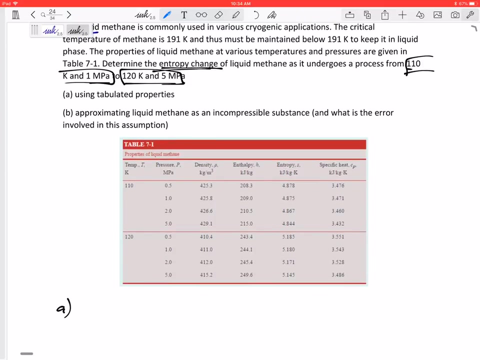 and 1 MPa to 120 and 5 MPa, using tabulated properties and then approximating liquid methane as incompressible and using the equation that we just derived up here, that I put with four stars for liquid methane. Alright, so for liquid methane properties, hey. 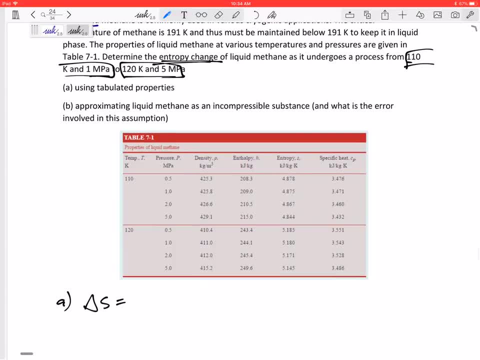 that's best, most accurate and sometimes easiest. Alright, it goes from 110 K and 1 MPa. Alright, so here is our S1.. Alright, there is our S1.. So S2 minus the change in S is S2 minus S1.. 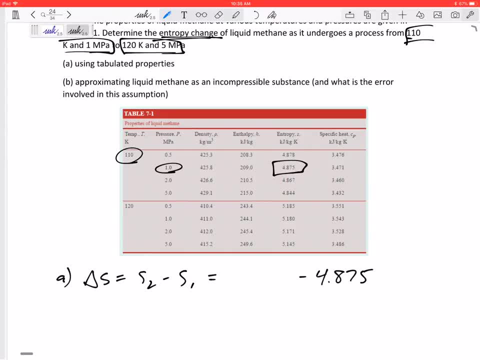 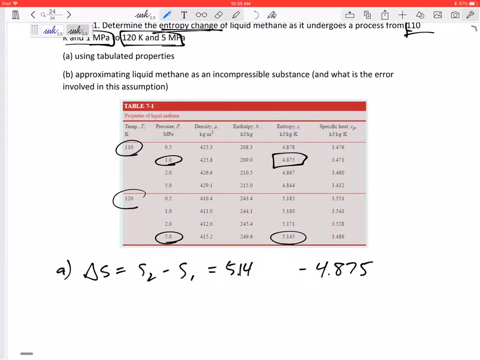 There's my S1.. 4.875 kilojoules per kilogram K. My final S2 is at 120 K, at 5 MPa, so down here 5.145. So the change in entropy is .270 kilojoules. 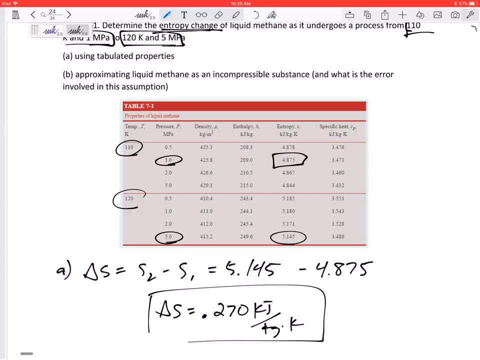 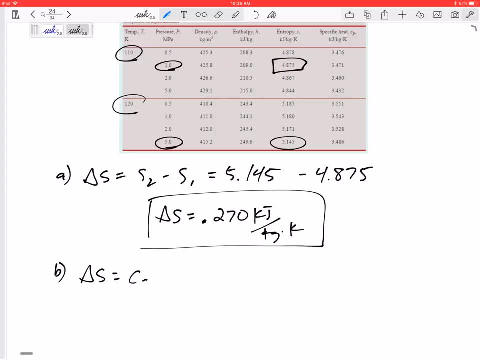 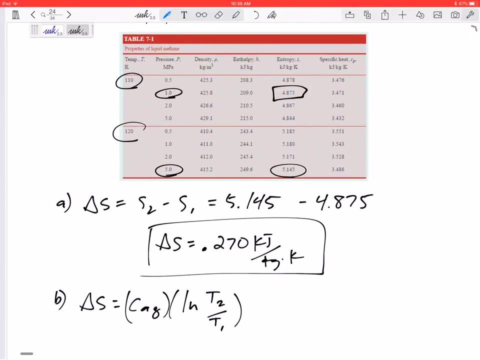 per kilogram K. Alright, that's most accurate. Now what if we wanted to use that equation? delta S is C average times ln, T2 over T1.. Alright, well, what is the C average? Um, well, the specific heat. 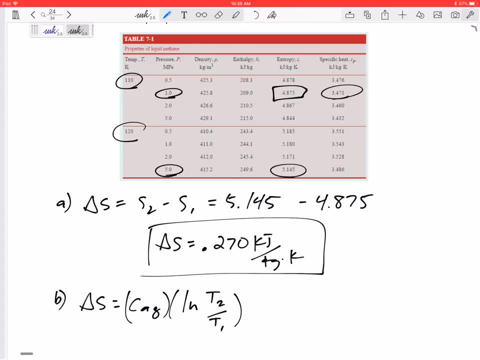 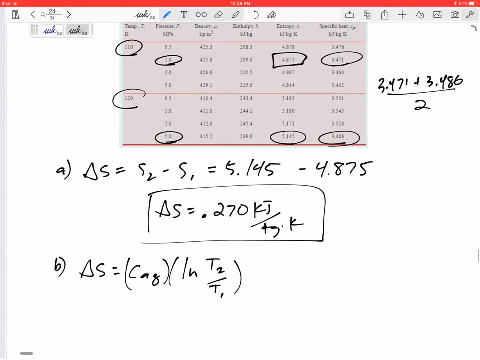 at the initial state is right there. The specific heat at the final state is right there. So the average of the two is 3.471 and 3.486 divided by 2. The average, I've got 3.4785. 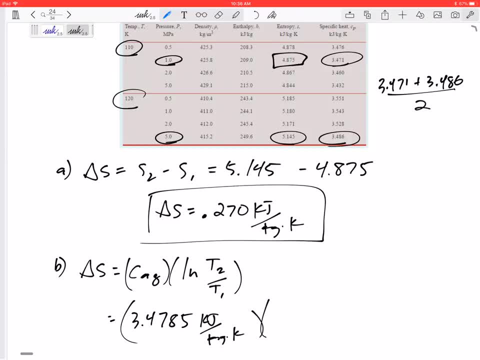 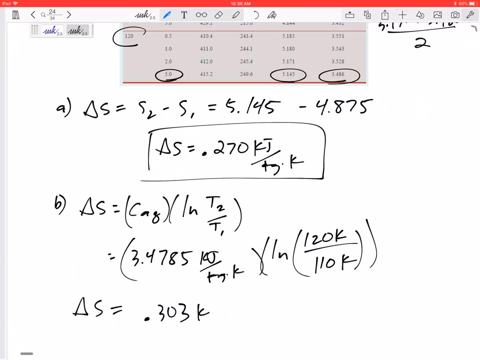 kilojoules per kilogram. K times ln, T2 over T1.. This these have to be in absolute temperatures. Of course. Kelvin is absolute temperature, so we're fine. So our delta S is .303 kilojoules per kilogram. 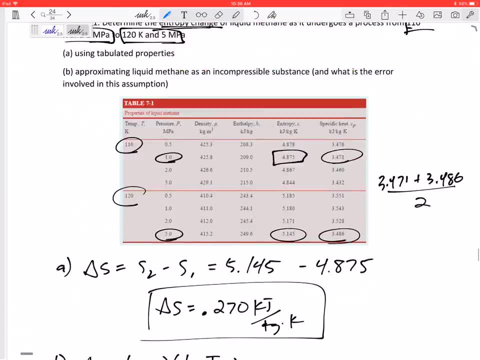 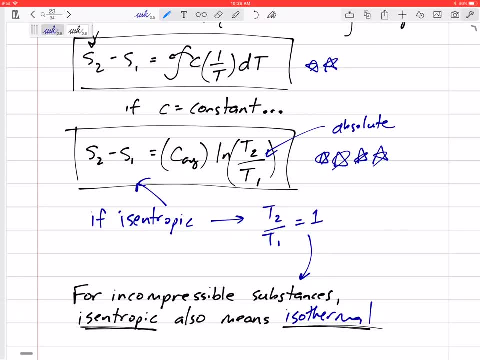 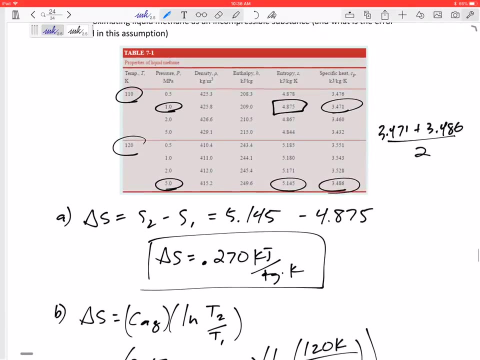 K. So there's my delta S right there. So just a note that up here this needs to be absolute. You would get different answers if you had those in Celsius. Alright, so there is the delta S, and what is the error in this assumption? 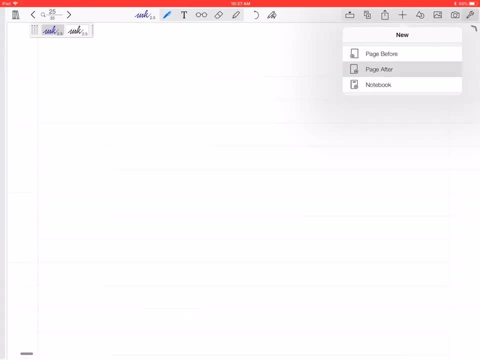 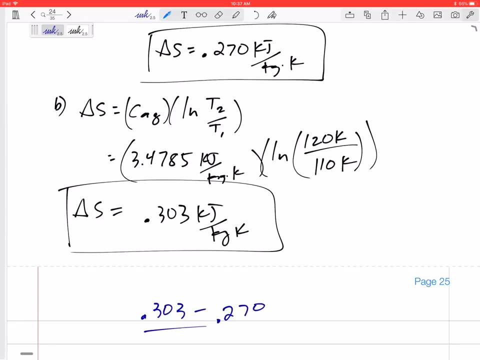 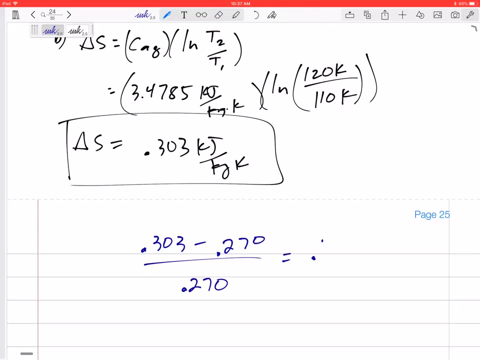 What's the error in this assumption? Well, what is the difference? What is the difference? Let's see .303 minus .270 divided by the original, .270 divided by the most accurate is .270 .122. So the error: 12.2.